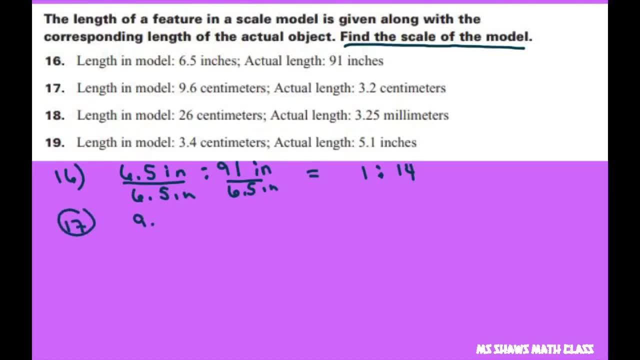 same thing: 9.6,. we're putting the model first, then the actual. So there's that 9.6 centimeters to 3.2 centimeters Divide both sides by 9.6.. Or let's just divide both sides by 3.. Let's divide it by the smaller number So it makes it easier: 3.2. And then that's going to give you 321.. That means the model is bigger than the actual. 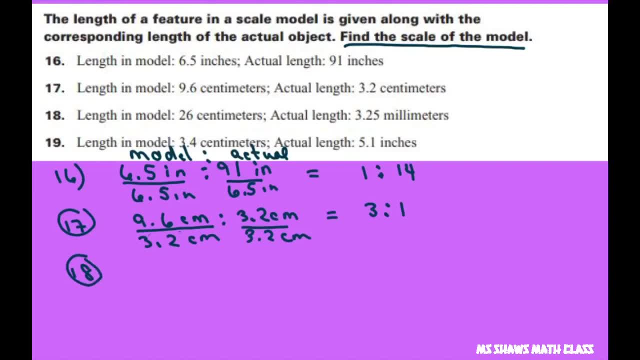 Then 18.. We have 26 centimeters to 3.25 millimeters. Now this one, we're just going to divide both sides by 3.25.. And you get 8.. And the way we're going to write it is 8. 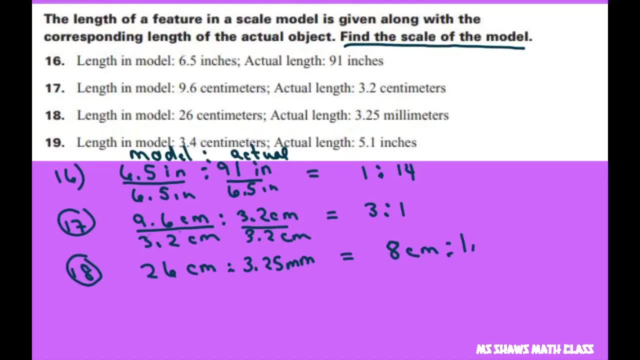 centimeters to 1 millimeter. So we're leaving our units in because we didn't convert units. And then for 19, do the same thing: 3.4 centimeters to 5.1 inches. So what we want to do is divide both sides by 3.4.. The smaller number gives you. we want it to be. 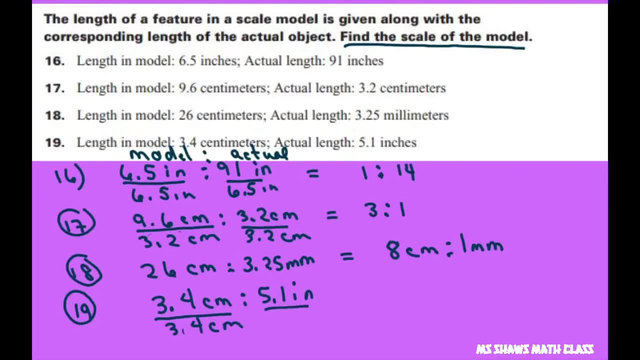 1 to something, And this is 3.4 inches, or just we're not doing centimeters- And then 5.1 divided by 3.4 gives you 1.5.. So this is going to equal 1 centimeter to 1.5 inches.